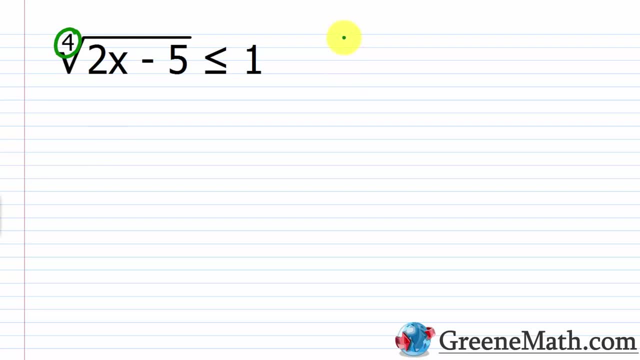 or something positive. So, when we set this up, the first thing we're going to do is we're going to set up a number. So we're going to take our radicand, which in this case is 2x minus 5, and we want to say that that needs to be greater. 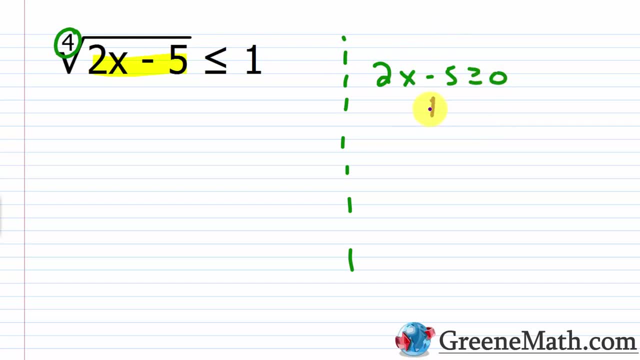 than or equal to zero. So I'm going to add 5 to both sides of this inequality and we're going to find that I have 2x is greater than or equal to 5.. Let me divide both sides by 2 and I'm going to. 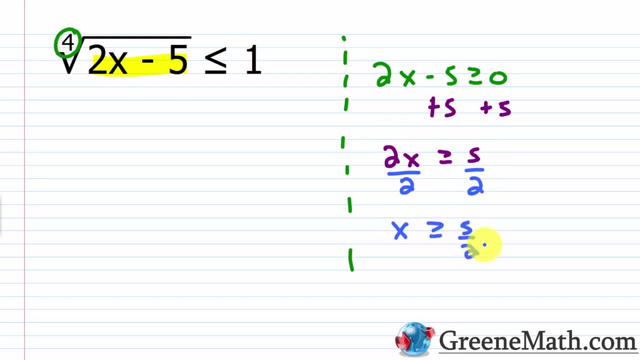 find that x needs to be greater than or equal to five halves. So in other words, if I plug in five halves for x, I will get zero there. right for my radicand, I can take the fourth root of 2x minus 0. that's just zero. That's okay. But if I plug in something less than five halves, I'm going to 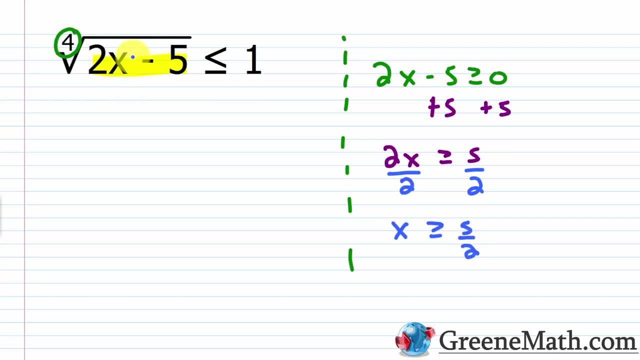 have a problem, right, because this guy, the radicand, wouldn't end up being negative. I can't, in the real number system, have the fourth root of a negative value because it doesn't exist. Okay, there's no number that I can raise to the fourth power and end up with a negative value because. 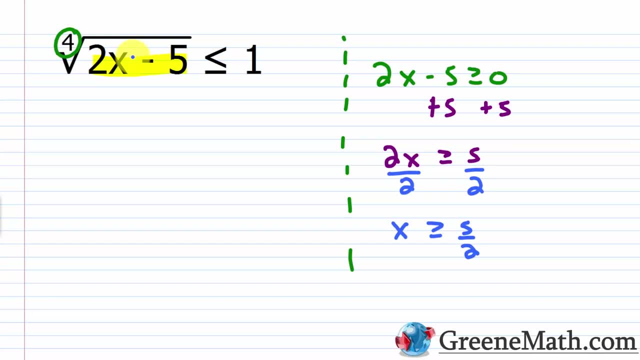 again, an even number of negative factors will always give you a positive result. Okay, so let me erase this, and I'm just going to write this up here. I'm going to write this up here. I'm going to write this up here. So we have that x is greater than or equal to five halves. Again, that's my 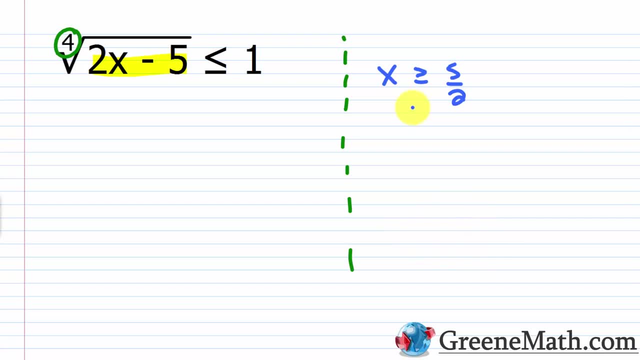 domain restriction. So the idea with this is: if I get a solution for my inequality and it violates the domain, I've got to reject it, Okay, so how do we solve the inequality? Well, one way that we can do this: we can replace the inequality symbol with equals and we can solve that to get our boundary. 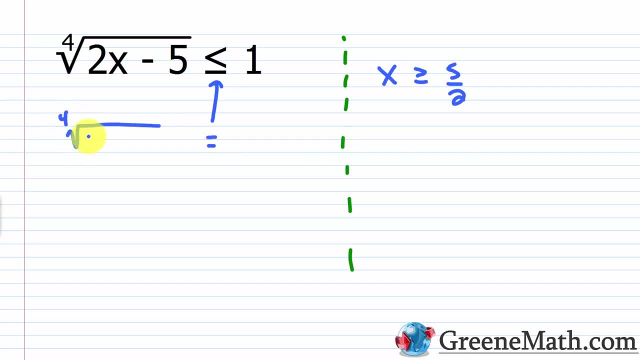 Okay, so we can say that we have the fourth root of 2x minus 5 and that's equal to 1.. Now that has to be 1 over 0 to get a value for 4 minus 1.. Now this equation, it's going to be very easy to solve. 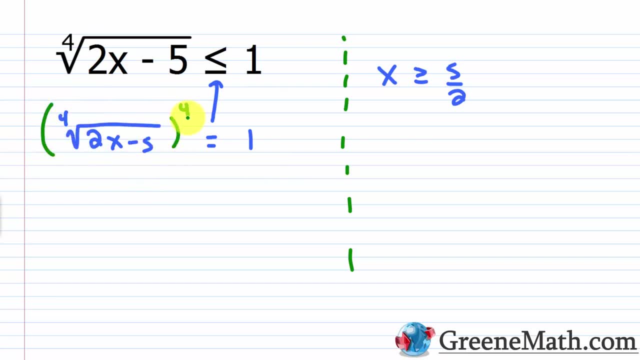 and I'm going to take morality. What I'm going to do here is I'm going to put mygrad cool, left, left. So to get rid of the radical, since my index is of four, I'm going to raise this to the fourth power and then, to make it legal, I'm going to raise this to the fourth power. So this is going to 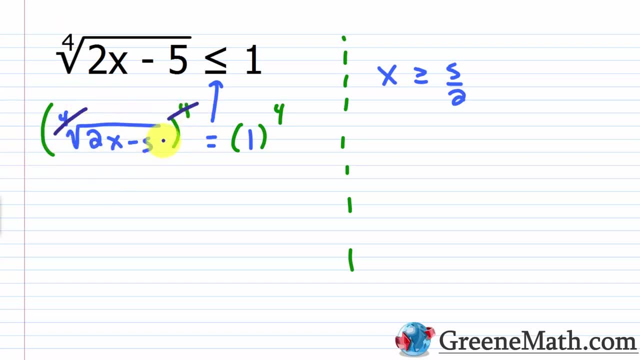 cancel here, and then I'm going to have my radicand right. So just my 2x minus 5, this will be equal to 1 to the 4th, power is obviously 1.. Now it's very easy to solve from this point. 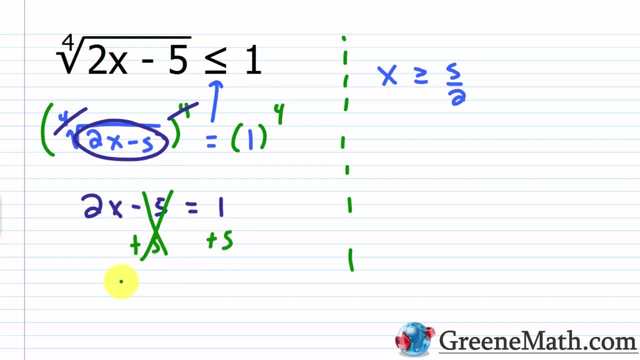 we just add 5 to both sides of the equation, so that's going to cancel and we'll get that 2x is is equal to 1 plus 5 is 6. one last step: we want to isolate X, so I'm going to divide both sides by 2 and we're gonna find that X is equal to 6 over 2 is 3. so 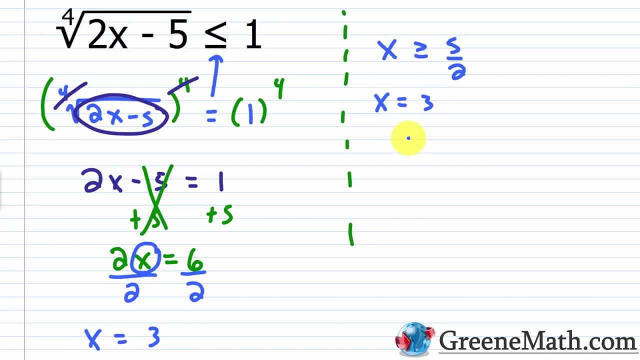 I'm gonna put X equals 3 here and that's gonna be my boundary, okay, so let's take these two values here down to the number line and we're gonna test a value on each side of 3. okay, 3 is the boundary, so I'm gonna test the value on the left. 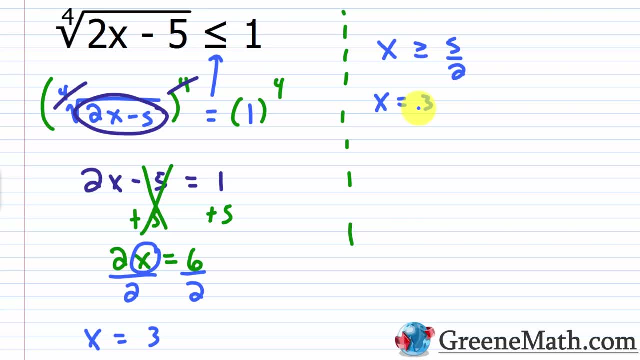 side of 3, something less than 3, and I'm gonna test something on the right side of 3, something greater than 3. but you have this restriction here. remember: X has to be greater than or equal to 5 halves, so we got to keep that in mind. so 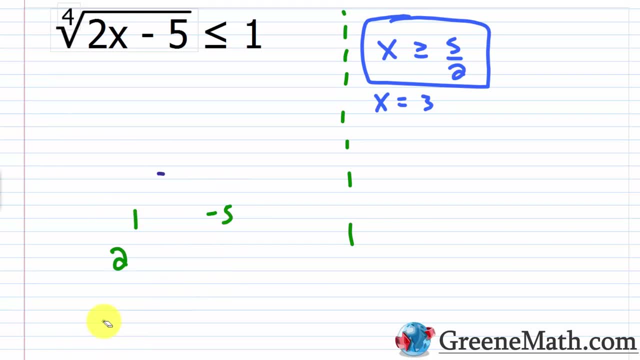 let's erase all this. and before I go down there, I want to show you one thing real quick. the first thing is that 3 works as a solution in this inequality. this is non-strict here. if I plug a 3 in 2 times 3 is 6. 6 minus 5 is 1, the 4th. 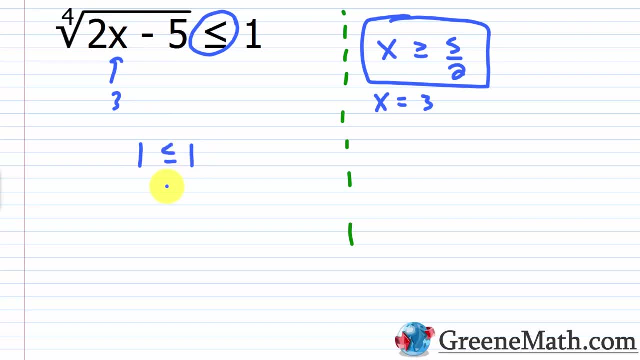 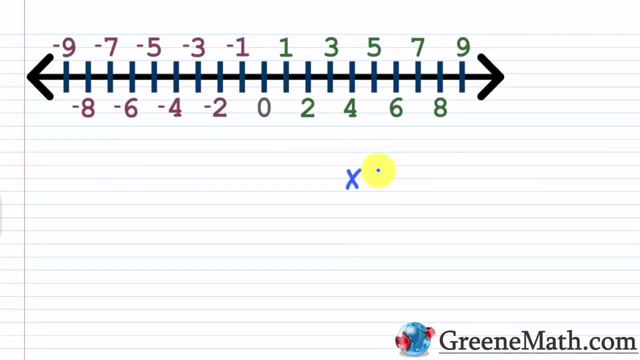 root of 1 is 1, so you get that 1 is less than or equal to 1, which is true. okay, so this guy right here works as a solution. so let's go down to the number line. so, again, our domain restriction is that X has to be greater than or equal to 5 halves, and then our boundary is: 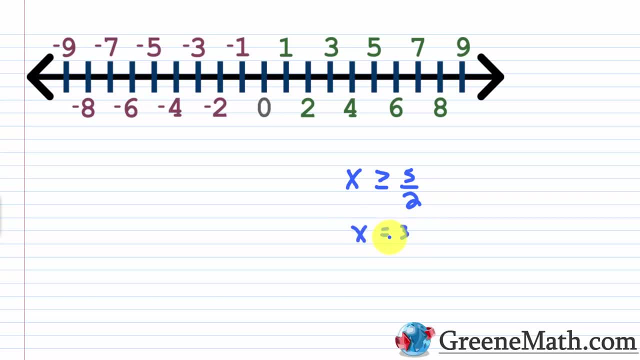 that X equals 3, which again works as a solution. so here's 3. let me put a vertical line there. and then 5 halves, as a decimal is 2.5. so let's put something right there and say this is 5 halves. so I can also put a vertical line there now. 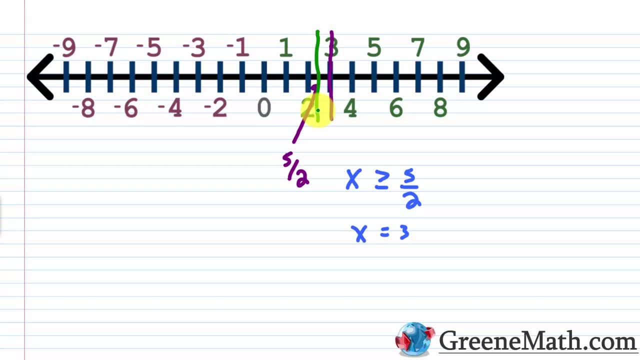 you can split this into regions, okay, this is very easy to do for reference sake. so, anything to the left of 5 halves, I'm just going to call that region a or interval a, anything between 5 halves and 3, and it's a tight window, I'm gonna call: 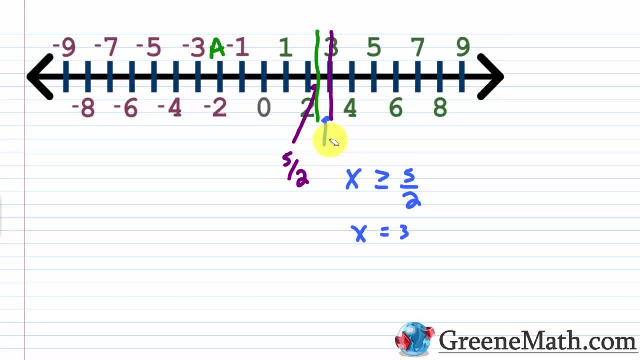 that interval B. okay, I'm just gonna put an arrow there because I can't really fit my letter there. and then anything to the right of 3, I'm gonna call that interval C. so for interval a, anything to the left of 5 halves- we know that's an. 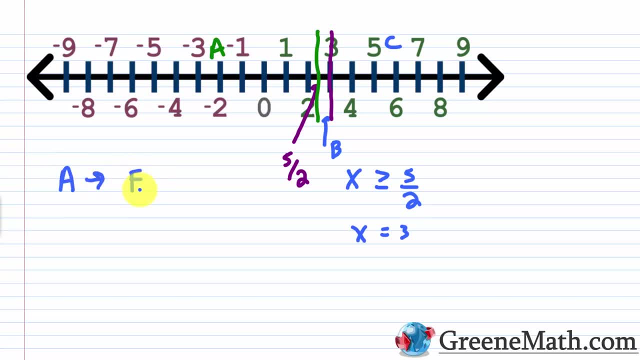 automatic rejection because it violates the domain. So I'm going to put an F there for false. Now for interval B, I need to test the value. So my original inequality was the fourth root of 2x minus 5 is less than or equal to 1.. So something between 2.5 and 3, I can do 2.75.. So let me get some room. 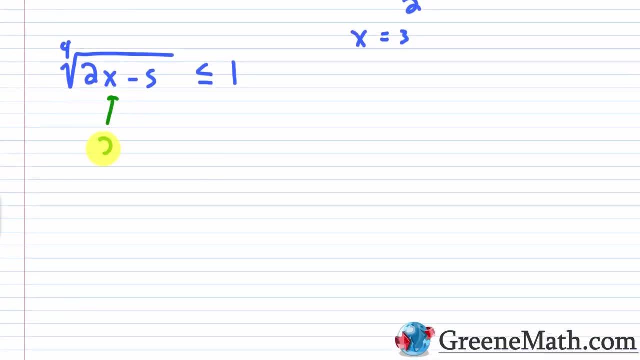 I'll come back up. So if I plugged in a 2.75 there for x, what would I have? I would have the fourth root of 2 times 2.75, which is 5.5.. So you'd have: 5.5 minus 5 is less than or equal to 1.. 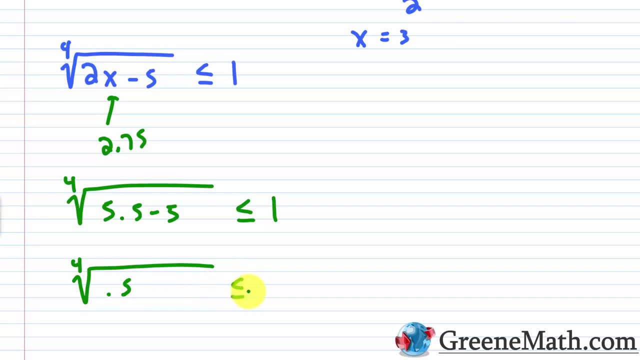 So then I have, the fourth root of 0.5 is less than or equal to 1.. Now, if I took the fourth root of 0.5, basically I can approximate that to be about 0.84.. Okay, about 0.84.. So if we had 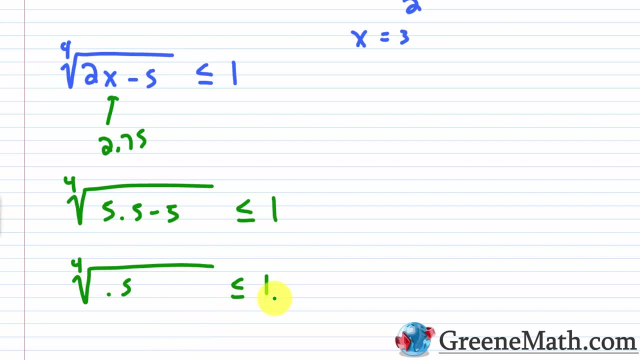 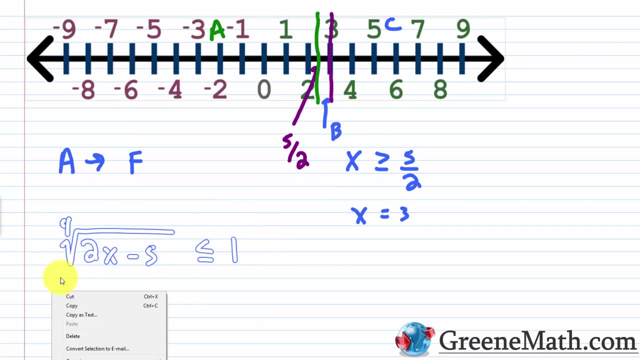 about 0.84,. that would be less than 1.. Okay, so that would be a true statement. So let me erase everything And I'm going to say that things in interval B work. Okay, let me slide this down just a little bit And I'm gonna put interval B right here And we'll 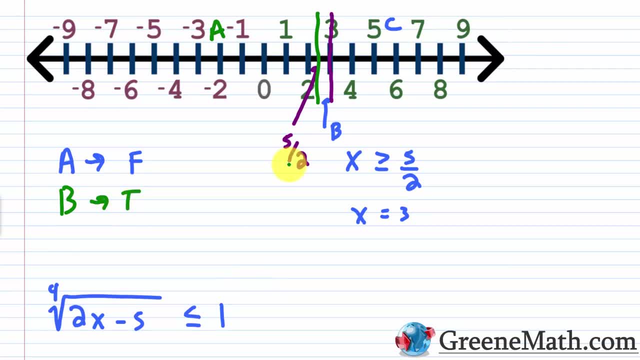 say that's true. Okay, so anything between five halves and three, including both. okay, three is included and five halves included, because essentially there's anything that's less than or equal to three. So it's going down to and including five halves because that's part. 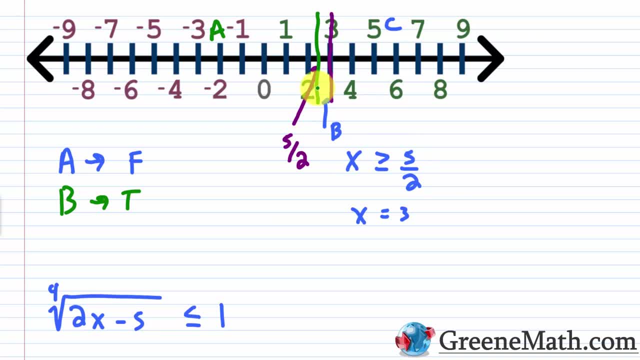 of your domain, But anything to the left of five halves isn't going to work because it's not. So what about things in interval C? so things that are greater than three? Well, you can test anything you want, So let's just pick four and plug that in Again. I'm just going to slide down. 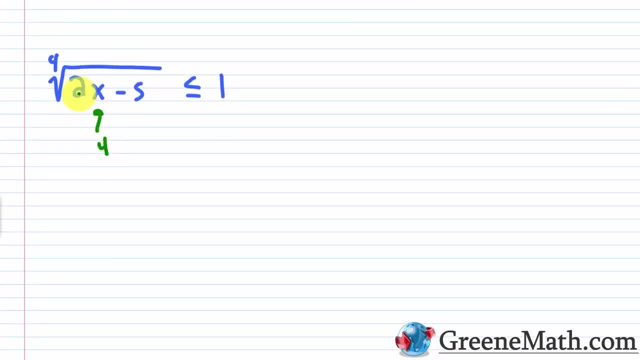 for a minute. So if I plugged in a four there, what would I get? Well, two times four is eight. eight minus five is three. So you'd have the fourth. root of three is less than or equal to one. So if 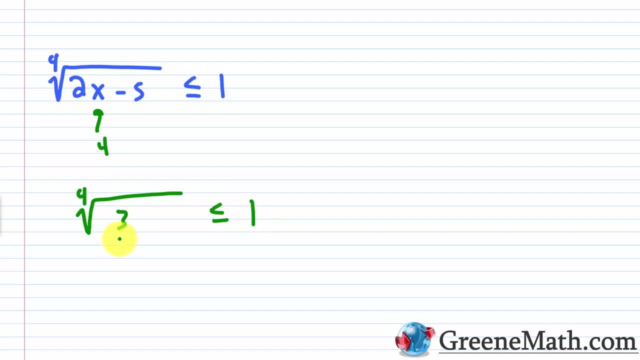 I approximate the fourth root of three, I'm going to get about 1.32, which is larger than one. Okay, so this is false. So this is false. So things in interval C don't work, And we'll say that for interval C. 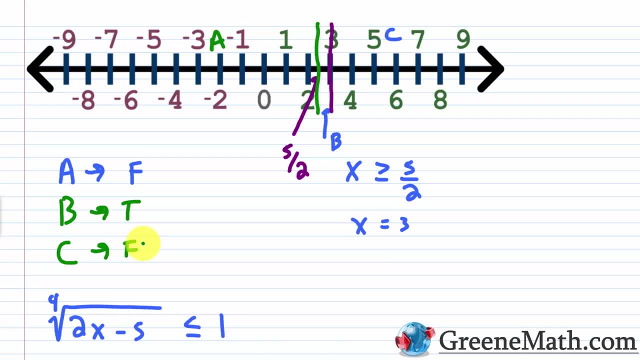 it's false. So I have my solution. Again, x is going to be any value, that's five halves and including five halves going up to and including the number three. So let me erase all of this. I don't need it anymore. So again, x is greater than or equal to five halves and less than, or: 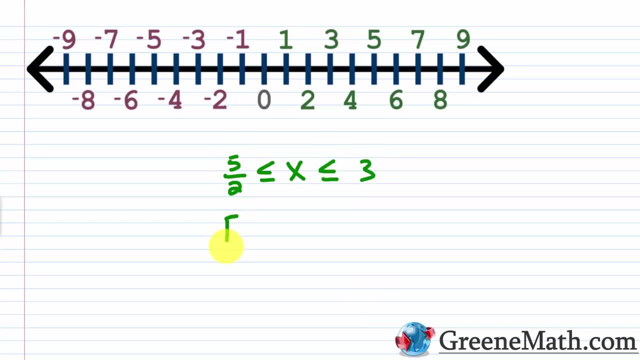 equal to three. Alright, so in interval notation I'm going to put a bracket next to five halves, Then comma, I'm going to put a bracket next to three And then, graphically again, let me put my 2.5 or my five halves back on the number line. So it's going to be right there. Again, this is my. 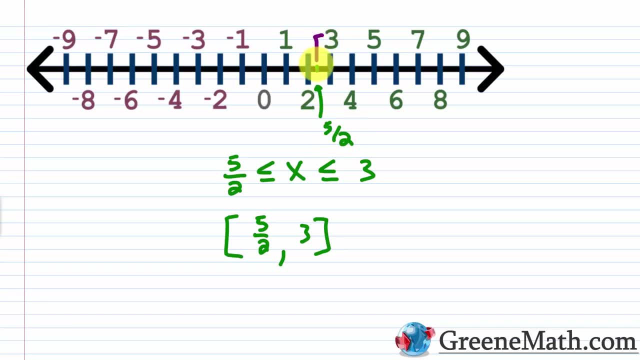 five halves. This is gonna be a tight window, but I'm going to put a bracket here. I'm going to put a bracket here. I'm just going to shade in between. So again, it's from five halves or 2.5. 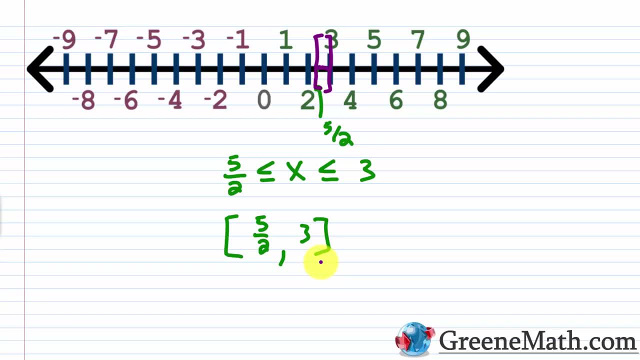 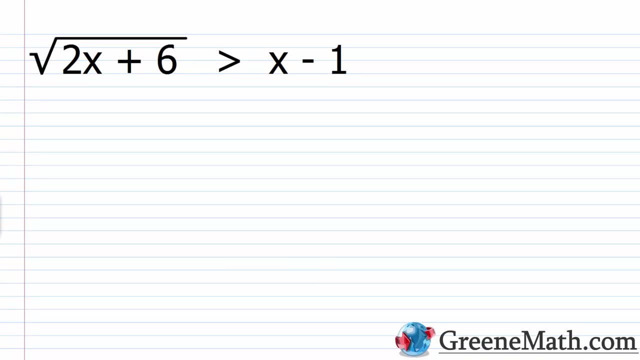 up to and including three. So the five halves is included and the three is included, and all the values in between. Alright, let's take a look at another one. So for this one we have the square root of 2x plus six. 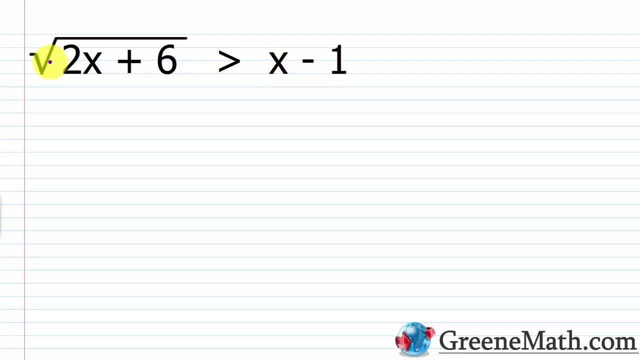 is greater than x minus one. Remember, if you have a square root involved, or again a fourth root, like we just saw, or sixth root, any even root, then you need to figure out what the domain restriction is going to be. So in this case, 2x plus six has to be set as greater than or equal. 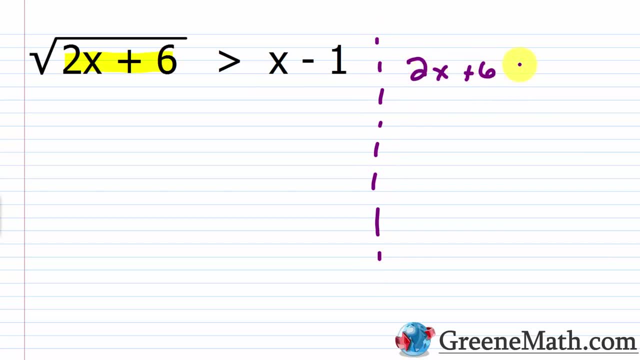 to zero, So 2x plus six. my radicand there again has to be greater than or equal to zero. So that's my domain restriction. Again, if I get something that's less than negative three, I've got to reject it. 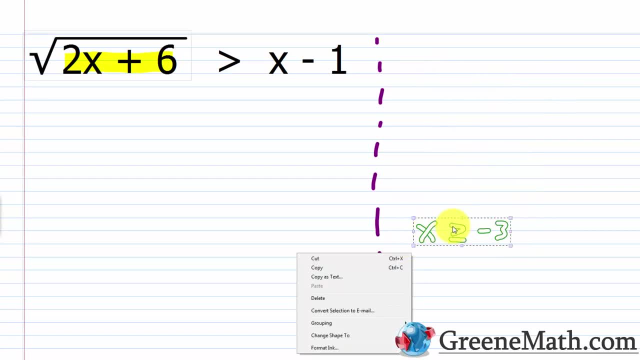 Okay, so let me go ahead and erase this and I'll slide this up. Now let's go about solving our inequality Again. the method I'm going to use: I'm just going to replace this with an equals and I'm going to solve the resulting equation. 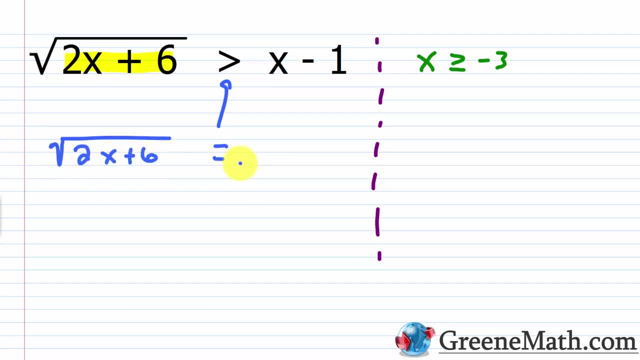 So we're going to have two x's and one minus one. So I'm going to have two x's and one minus one. I'm going to have the square root of 2x plus six is equal to x minus one. So again, the radical on the left. 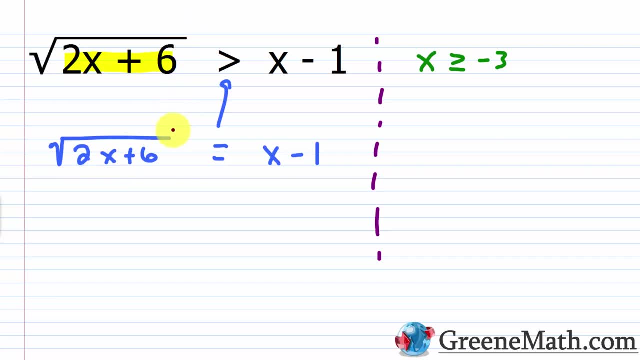 side is already isolated, So I can go ahead and just square both sides. So I'm going to square this side and I'm going to square this side. So what's going to happen over here is this is going to cancel with this. I'll just have my radicand. So the left is 2x plus six On the right side. 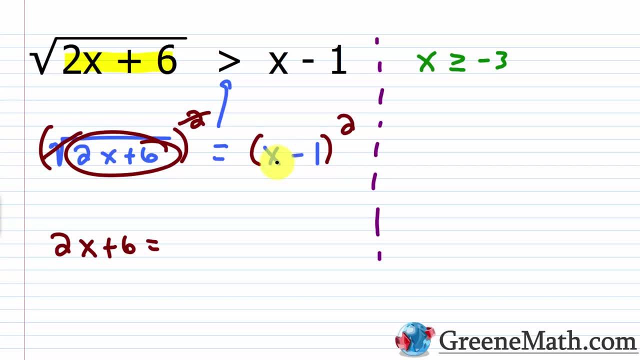 remember I have to expand this. Okay, so x minus one, that quantity squared, you can use your formula: It's the first guy squared, So x squared, then you have a minus there. So it's going to be minus two times this guy times this guy. So two times x times one is 2x, Then plus the last guy, one. 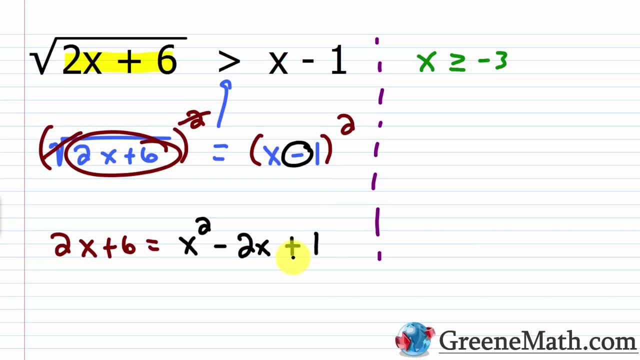 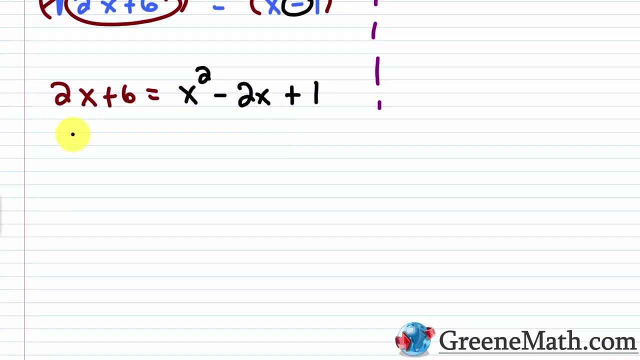 squared, So plus one. Okay, so what I'm going to do, since I'm going to end up with a quadratic, I'm just going to go ahead and move everything on the left over to the right, So my left is going to. 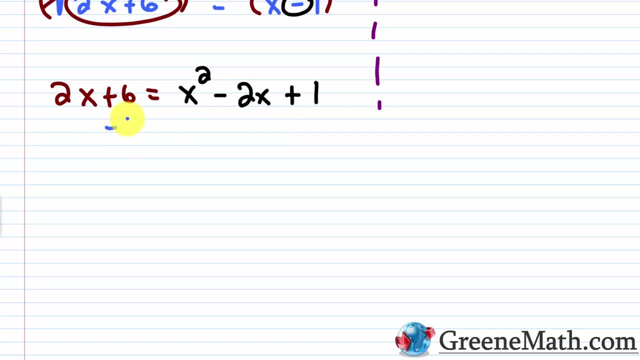 be zero. Okay, so what I'm going to do? I'm going to subtract six away from each side of the equation. That's going to cancel. And I'm going to subtract 2x away from each side of the equation, So that's going to cancel. So the 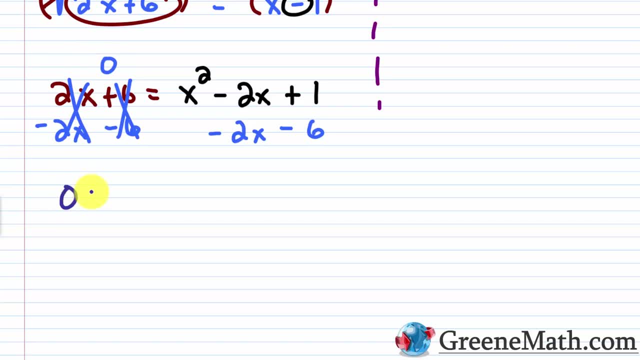 left side is now zero, So I'm going to have that zero is equal to x squared negative. 2x minus 2x is minus 4x, And then one minus six is going to be minus five. So you can flip this around if you. 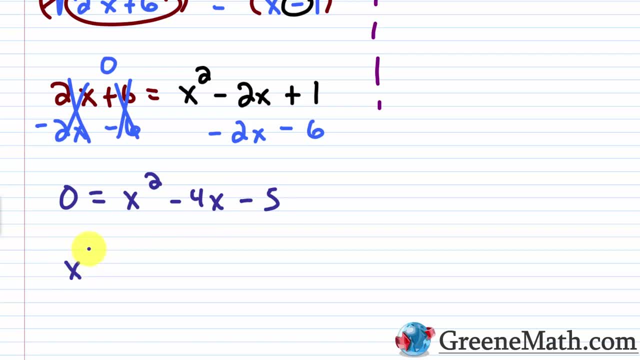 want. I know most of you, including myself, like the variable parts on the left. So you can say: x squared minus 4x minus five is equal to zero. That's perfectly legal. Let me scroll down a little bit more. This is one that we can solve using factoring. So that's what I'm. 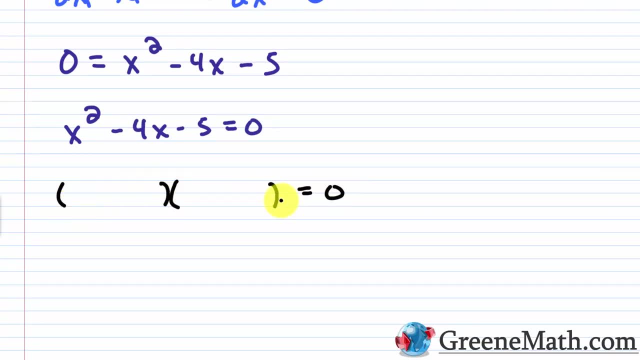 going to do For the left side. I can factor that by putting an x here and an x here, And they give me two integers whose sum is negative four and whose product is negative five. Well, negative five can only come from one times negative five, or negative one times positive five. So what I'm? 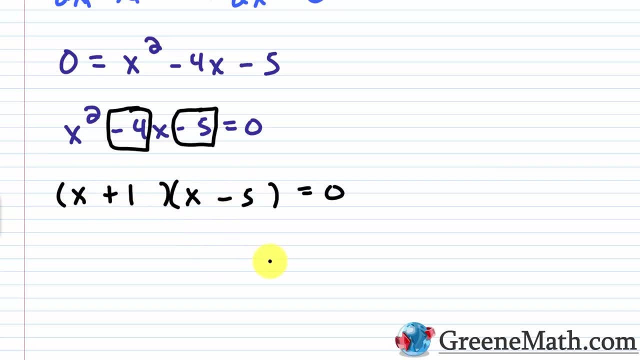 looking for is positive one and negative five. So if we solve this using our zero product property, we're going to have x plus one equal to zero. Of course, that would give us a solution of x is equal to negative one, And we would set x minus five equal to zero, And that would give us a solution of 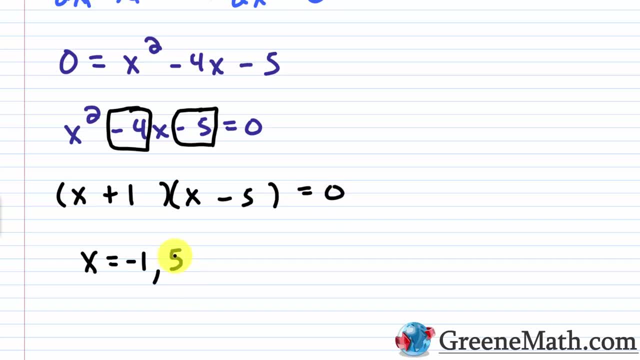 positive five. Now one of these is going to be extraneous. Okay, so let me erase everything. We're going to check both of these and I'll show you which one's extraneous. All right, so again, we found that the solutions for this equation are: x equals negative one and five, If you plug in a. 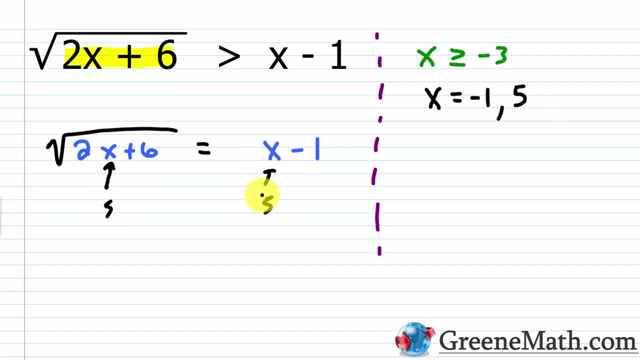 five, you're fine. So if I plugged in a five there and also there, I'd be okay. Two times five is 10.. 10 plus six is 16.. The square root of 16 is four Over here. 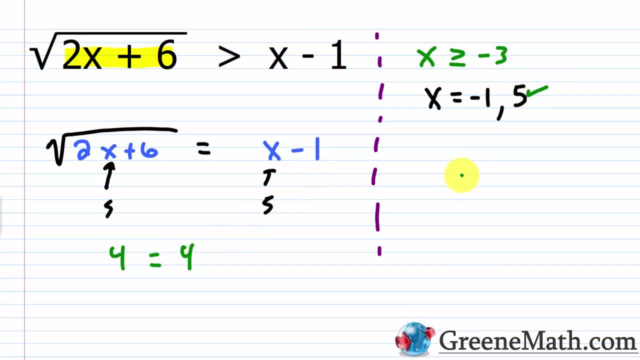 five minus one is four. So this one is good to go. But with negative one you're going to have a problem. Okay, with negative one you have an issue. You plug that in here and here Two times: negative. one is negative two. Negative two plus six is positive four. So you'd have the square. 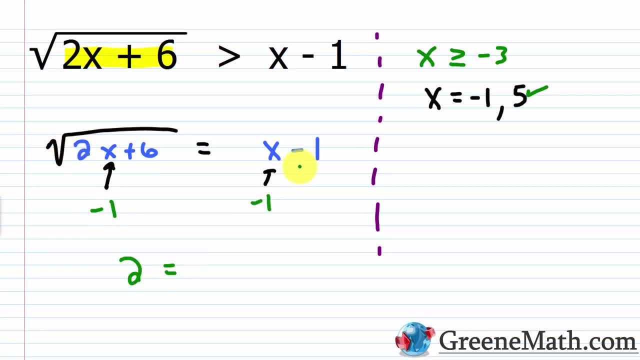 root of four, which is two, And that's equal to negative. one minus one is negative two. So obviously this is false. Okay, this is false, It's an extraneous solution. So your boundary here is five And basically your restriction is: 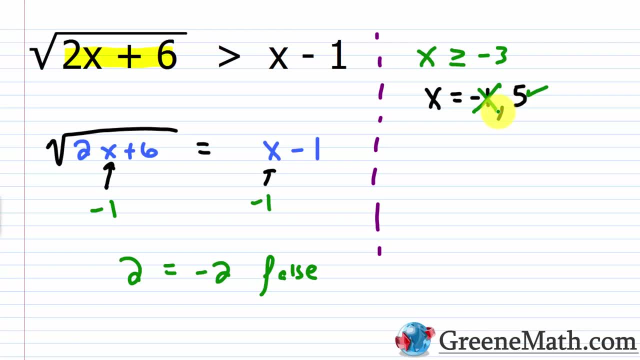 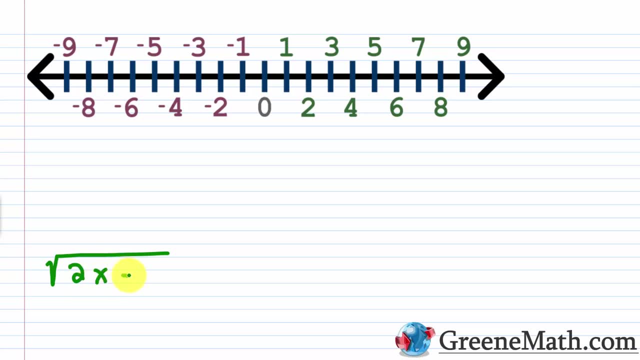 that x needs to be greater than or equal to negative three. So let's take this information down to the number line. So again, my inequality is the square root of two x plus six, And again this is greater than x minus one. My restriction on the domain is that x needs to be greater than. 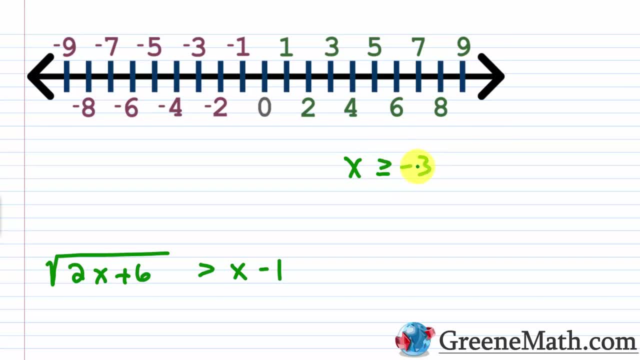 or equal to negative three, And my boundary occurs at five. So x equals, five is the boundary. So on the number line, five is here, should draw a vertical line there And negative three is here. So let's draw another vertical line here. So we know anything to the left of negative three. doesn't work, So let me go. 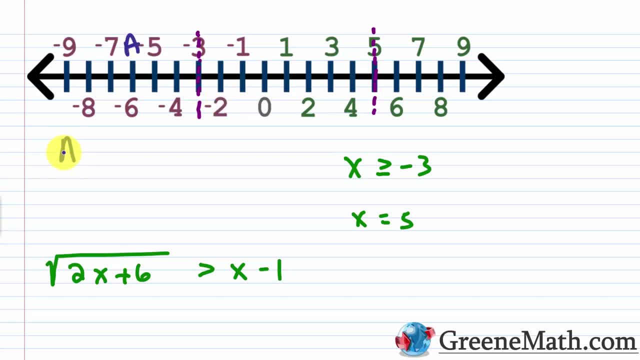 ahead and put this as interval a again, anything to the left of negative three, And I'm just going to put that this is an automatic rejection, right? So an F for false. then you have anything between negative three and five. So this area will be called b and this one will be called c. Okay, so let's start out by testing. 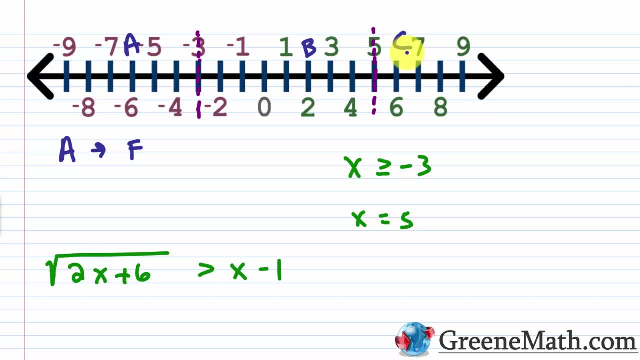 something in interval b. So again, this is between negative three and positive five. So if I plugged in, let's say I don't know how about zero? So let's plug that in there and there and see what we get. 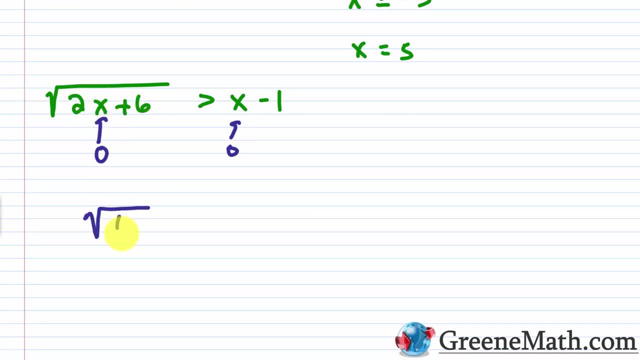 So we know that two times zero is zero. So you have, basically: the square root of six is greater than zero minus one is negative one. Well, we don't need to know what the square root of six is, We don't need to even approximate it, because this is a positive number. Of course it's going to be. 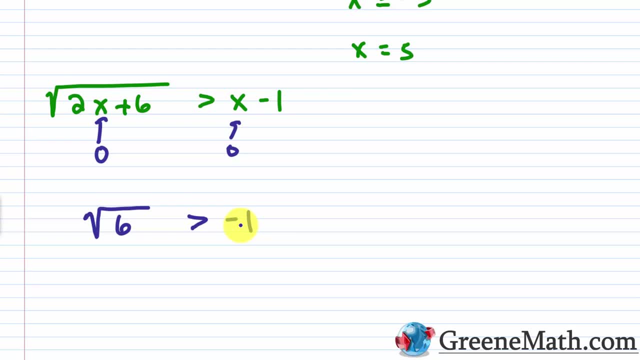 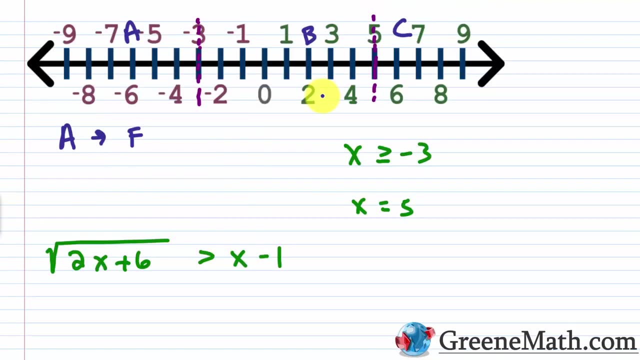 greater than a negative one, because a positive number is always greater than a negative. Okay, so this is true. So let me erase this. We'll basically say that things in interval b will work. So for interval b, it's going to be true. So it's going to be anything that's less than five. 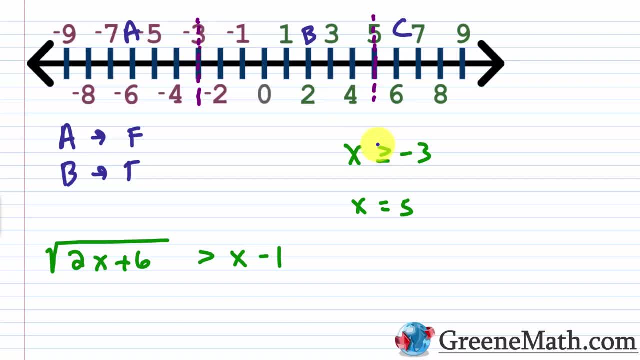 going down to and including negative three, because negative three is still in the domain. Okay, Now what about things in interval c? Do they work? To make this easy on ourself, let's choose 29.. So I could plug that in for x there. 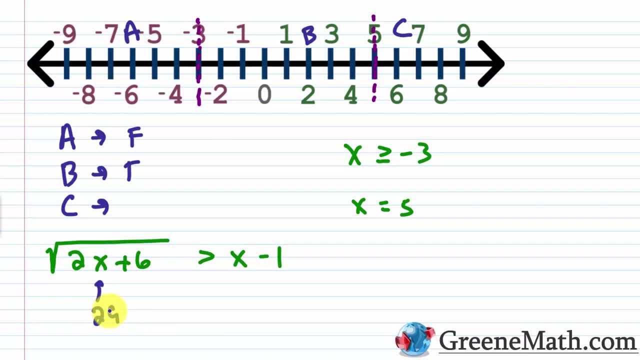 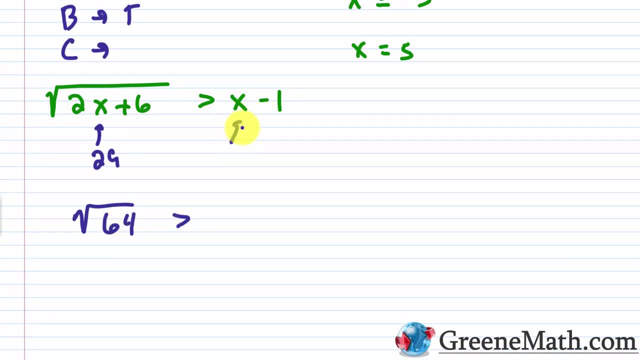 Two times 29 is 58. Then if I add six, I get 64. So what you'd have is the square root of 64 is greater than 29 minus one, which is 28.. I know the square root of 64 is eight. Eight is not greater. 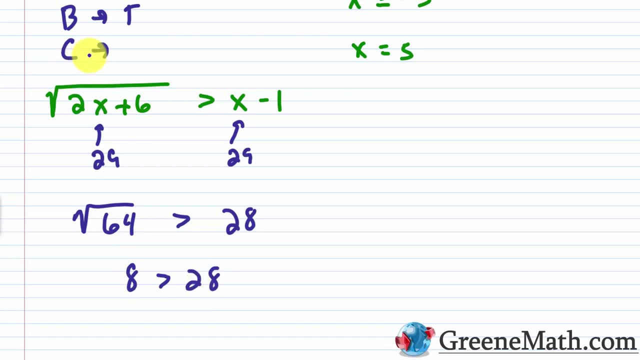 than 28.. That is a false statement. So things in interval c will not work. So I'll put an F there and I'm going to put a negative three. Okay, So I'm going to put an F there and I'm going to put an F there. 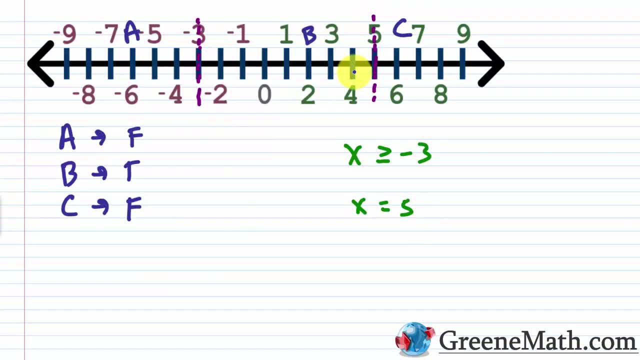 So I'm going to put an F there, and I'm going to put an F there, and I'm going to put an F there, All right, So we have our solution now. So anything in interval b will work. So again, we've got to be specific here. It's anything less than five, but because we have this domain, 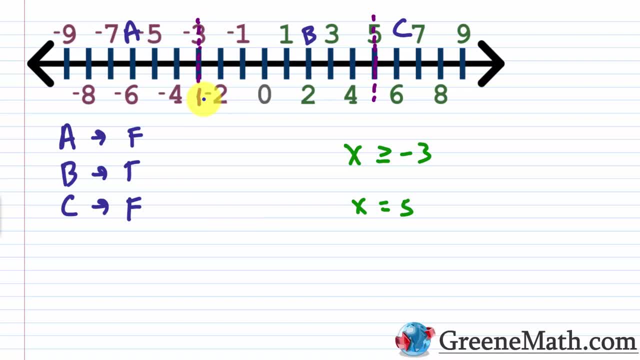 restriction that anything less than negative three doesn't work. you're basically say that x has to be greater than or equal to negative three, but less than five. Okay, So negative three is included. Five is not All right. So in interval notation I can say that again. 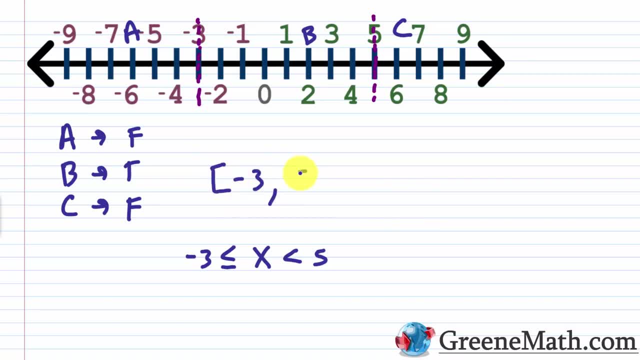 negative three is included. by putting a bracket there And then comma, you have a five and then a parenthesis And then graphically erase this. So again, at negative three, I'm going to have a bracket, At five, I'm going to have a parenthesis. 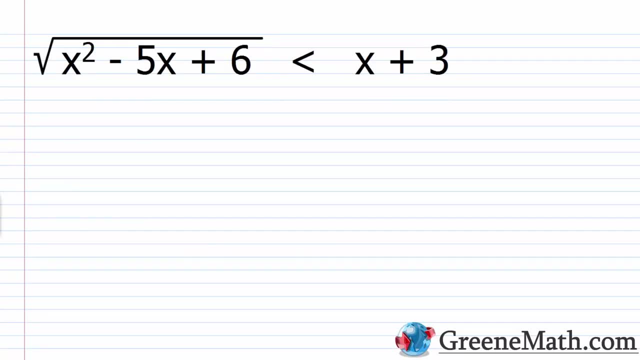 I'm just going to shade everything in between. All right, Let's take a look at one to wrap up the lesson. that's pretty tedious. So we have the square root of x squared minus five. x plus six is less than x plus three. So what makes this problem tedious is that you have a quadratic. 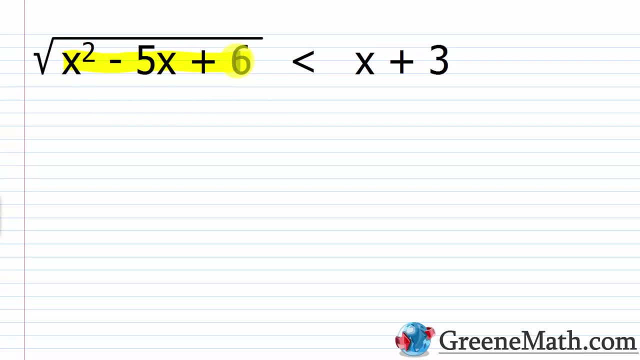 inequality that you're going to need to set up to figure out how to solve this problem. So we're going to need to find your domain restriction right, Because you have x squared minus five, x plus six. That's underneath the square root symbol, So we need to set this as. 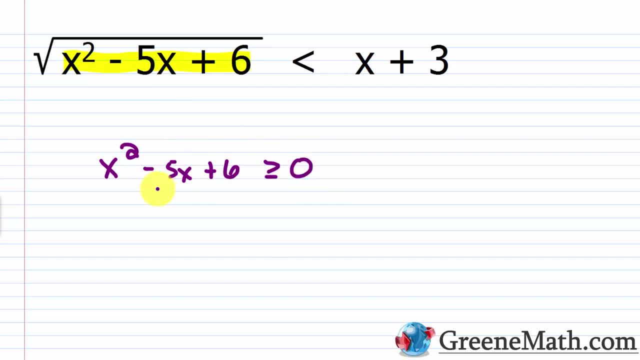 greater than or equal to zero. Okay, So this guy right here. again, it's a quadratic inequality. At this point, we know how to solve this. We're going to replace this guy right here with equals And we're going to solve: x squared minus five, x plus six equals zero. This will give us our 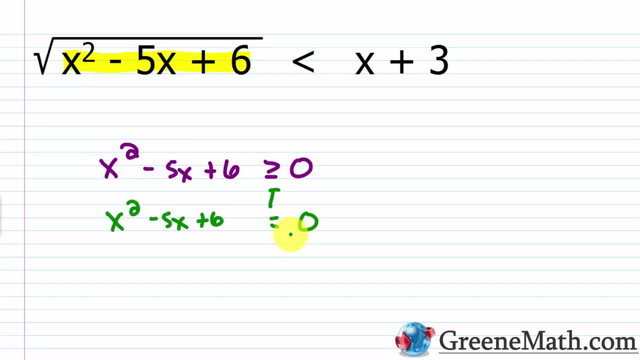 boundary or, again, critical values, And then we're going to solve this guy right here with equals, And then we're going to test values on each side of that. Okay, So we're going to set up intervals and test, just like we've been doing. So what I'm going to do is solve this by factoring. 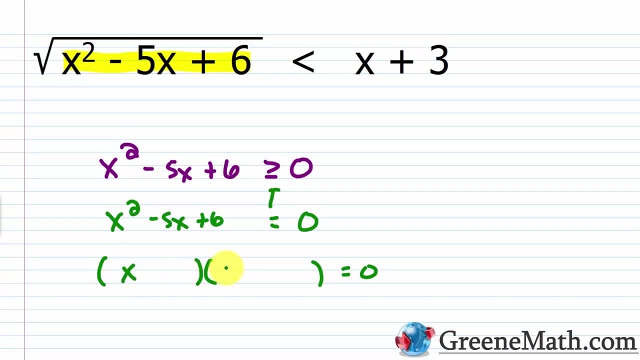 I know that this guy would be x and this guy would be x. Two integers that sum to negative five and give me a product of positive six would be negative two and negative three. right, Negative two plus negative three is negative five. Negative two times negative three is positive six. 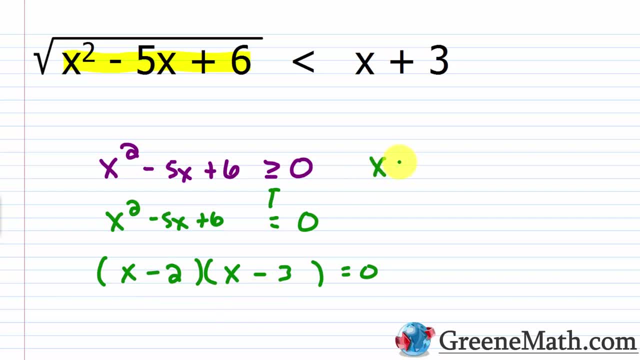 So if I solve this equation, I would find that x is equal to x squared minus five. x plus six. Negative three is equal to y. X minus two is equal to zero. That has a solution of x equals positive two. If x minus three is equal to zero, that has a solution of x equals three. Okay So. 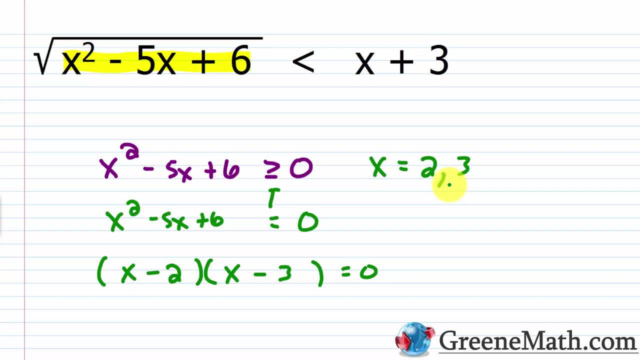 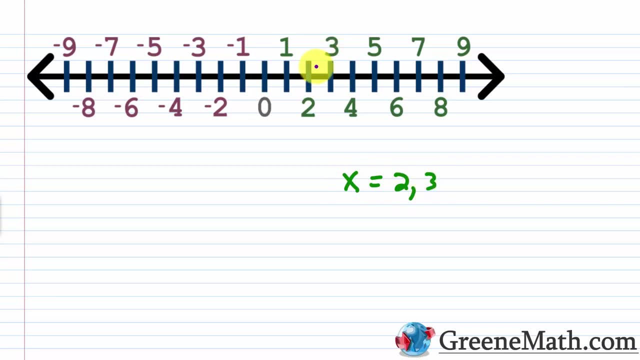 two and three are going to be my boundaries. So let's go down to the number line. So again the critical values or the boundaries. x equals two and three. So here's two, here's three, And again we're going to set up intervals. So anything to the left of two is a. 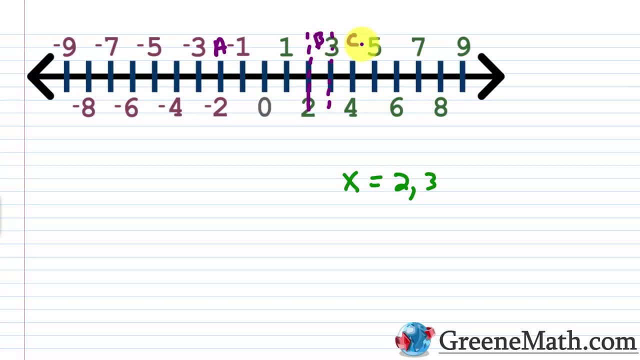 anything between two and three will be b. anything between two and three will be b. So we're going to set up intervals. So anything to the left of two is a And anything greater than 3 will be C. So again you've got A, B and C. 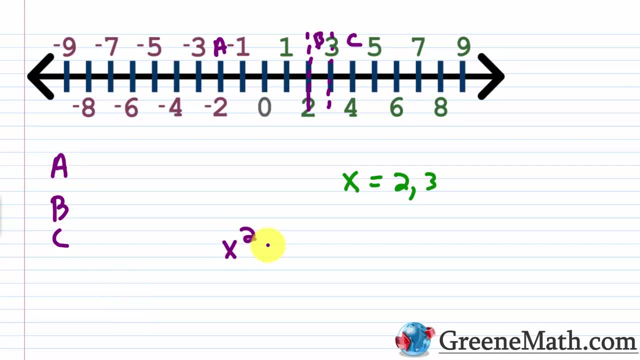 So let's test some values. So again we've got x squared minus 5x plus 6 is greater than or equal to 0.. So let's start out by testing 0.. That's something in interval A. We know that that would basically mark out this guy and this guy. 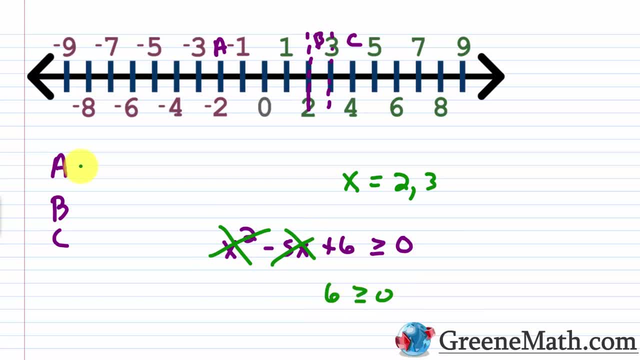 So it would have: 6 is greater than or equal to 0, which is true. So for interval A, things work, That's true. What about interval B? Well, I can take something like 2.5. That's between 2 and 3.. 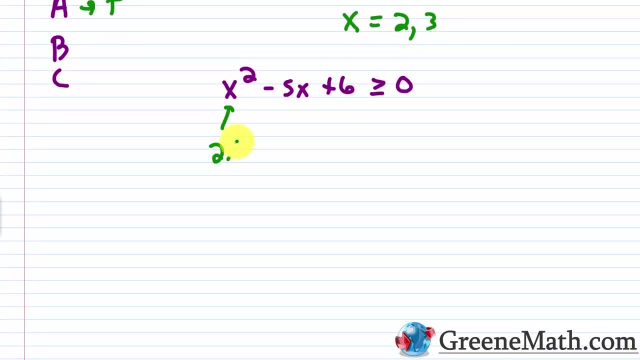 So 2.5.. So if I plugged in a 2.5 there and there, what would I get? Well, 2.5 squared is 6.25.. Then if I subtract away 5 times 2.5,, 5 times 2.5 is 12.5.. 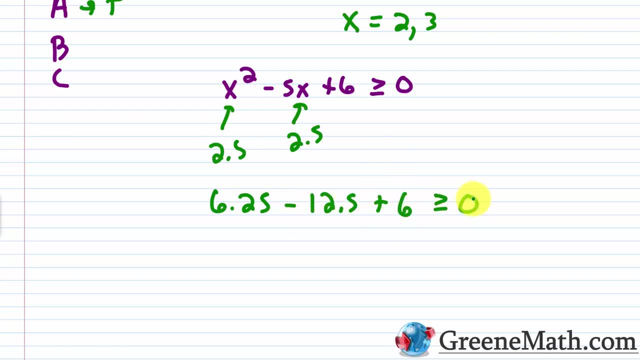 Then if I add 6, is this greater than or equal to 0?? Well, no, it's not, Because 6.25 plus 6 is going to be 12.25.. So 12.25. And if I subtract away 12.5, I'm going to get negative. 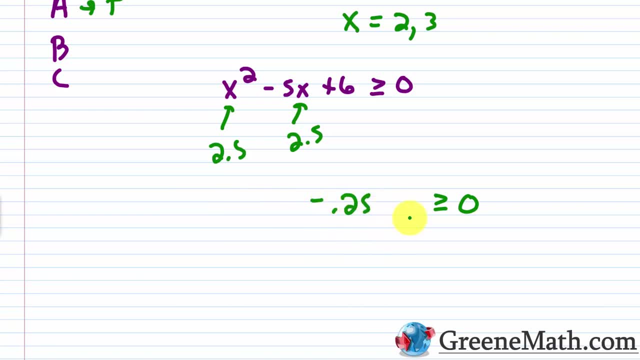 I'm going to get negative 0.25.. So that's not greater than 0 and it's not equal to 0, because obviously it's a negative, and so it's not going to be greater than 0.. Okay, so let's erase this. 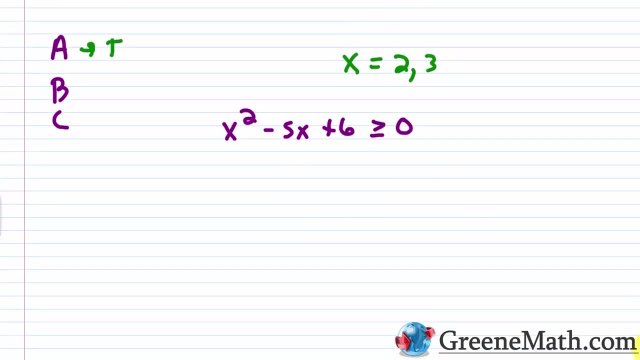 We're going to say things in interval B don't work. Okay, so let's go back up, And so we'll say things in interval B again, between 2 and 3, those don't work, So that's going to be false. 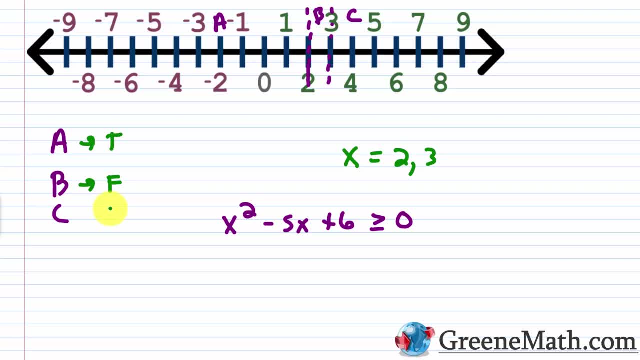 Then, lastly, let's check something in interval C. So let's just pick 4.. That's easy to work with, So I'll plug in a 4 there and there. So 4 squared is 16.. And then, minus 5 times 4 is 20.. 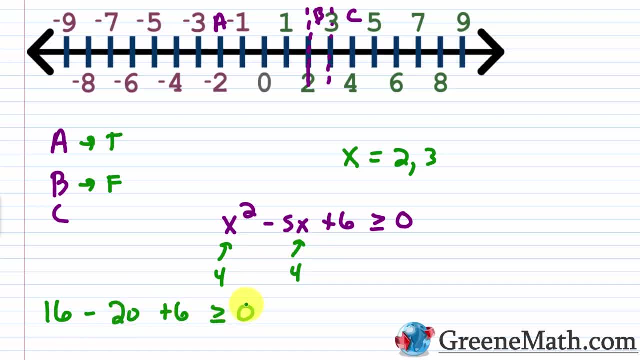 And then plus 6, is this greater than or equal to 0?? Well, 16 plus 6 is 22.. 22 minus 20 is positive 2.. So you'd have that 2 is greater than or equal to 0, which is true. 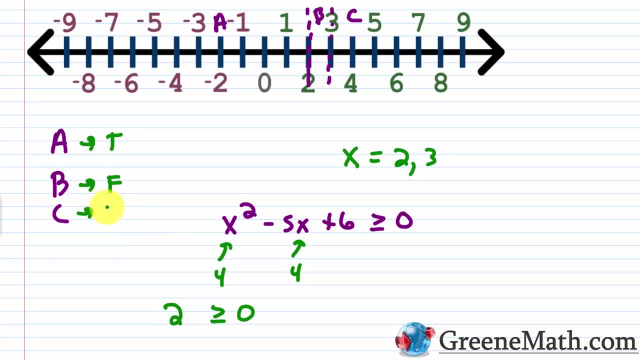 So for interval C or region C or whatever you want to call it, this is going to be true. So I've found my domain. Okay, I've found my domain. Basically, we can say that x needs to be 1. It needs to be greater than or equal to positive 3.. 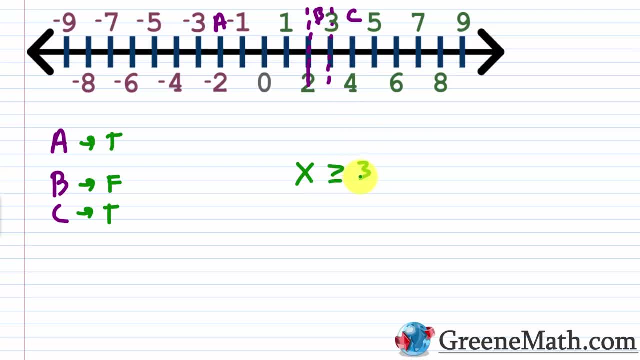 And the or equal to is because I had a non-strict inequality, So the endpoints or the boundaries are going to be included Then, or x needs to be less than or equal to that value of 2.. So the values that don't work in our inequality are going to be things between 2 and 3.. 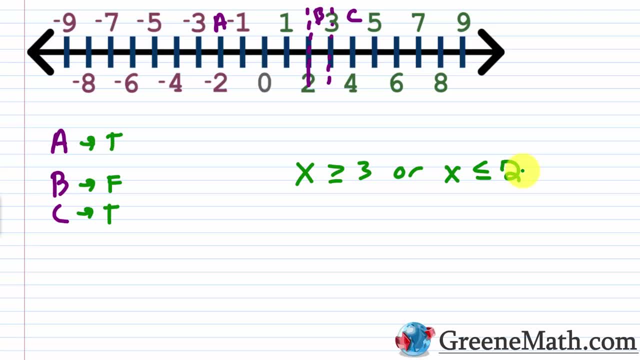 2 works, 3 works, But it's got to be less than 2 or equal to 2, or greater than 3 or equal to 3.. But anything in between will not work. So I'm going to leave this here, because we're going to work on this later on. 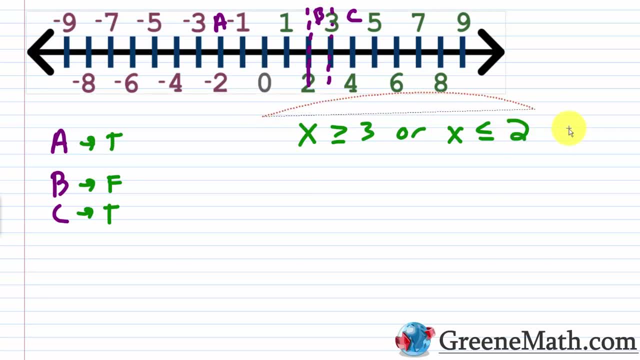 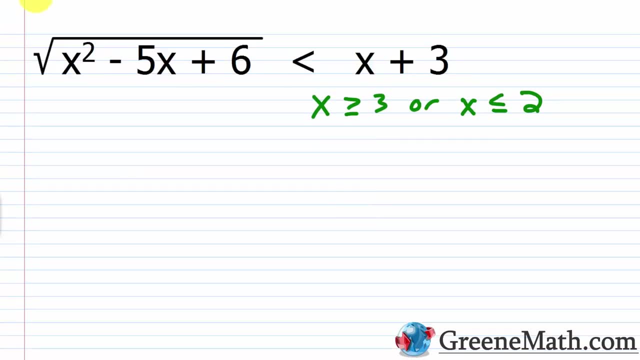 So this will just stay here, But I'm also going to copy it and bring it up for reference sake. We're done with this information. We can erase it. So to solve the inequality. now I know my domain. I'm just going to replace that with equals. 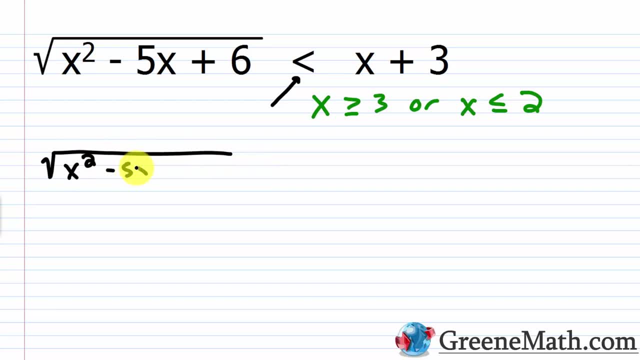 So I'm going to have that the square root of x squared minus 5x plus 6. Is equal to x plus 3.. So to solve this, my radical is already isolated on the left, So I'm just going to square both sides. 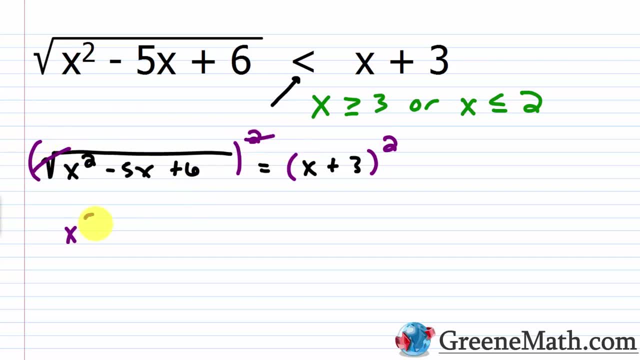 So this is going to cancel with this And I'll have my radicand of x squared minus 5x plus 6.. And this is equal to- again, you've got to expand this. So this is going to be x squared plus 2 times x times 3,, which is 6x, plus 3 squared, which is 0.. 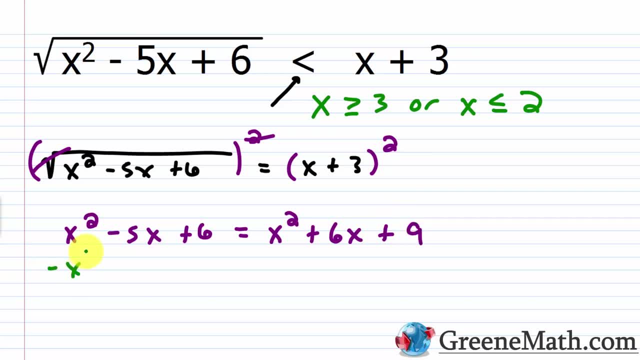 Now I have x squared on each side. I can subtract that away From each side Again. if you see the same thing on each side, you can just get rid of it. So I can cancel this and this. So on the left side I have negative 5x plus 6.. 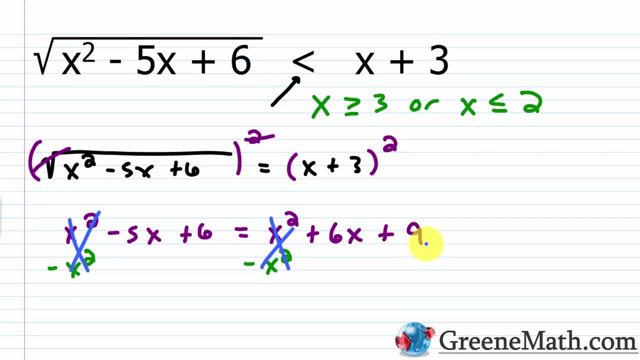 On the right side I have 6x plus 9.. So let's move all the variable terms to one side, all the numbers to the other. So let me subtract 6 away from each side And let me subtract 6x away from each side. 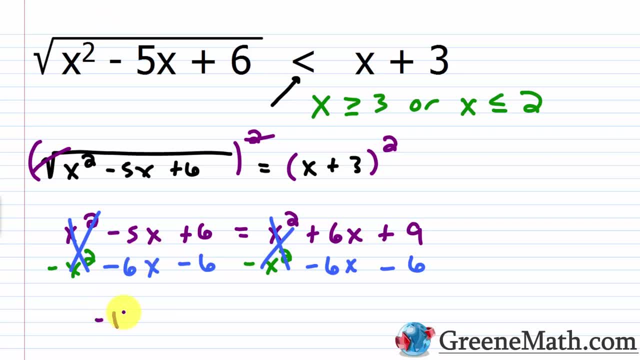 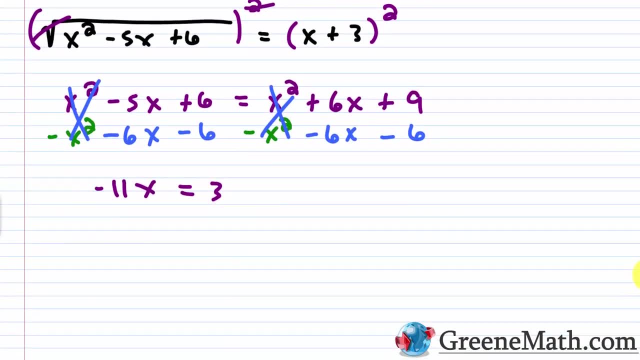 So negative 5x minus 6x is negative 11x. This is equal to over here: 9 minus 6 is 3.. So to get my solution for x, I'm going to divide both sides by the coefficient of x, which is negative 11.. 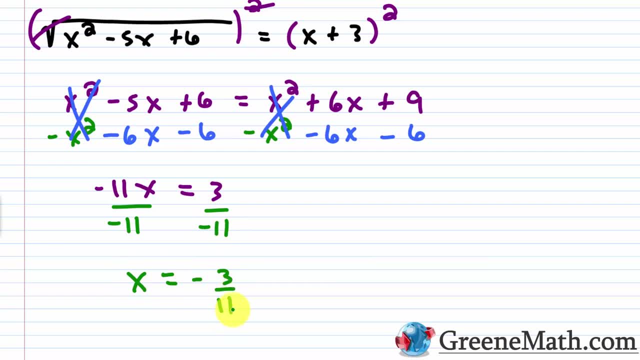 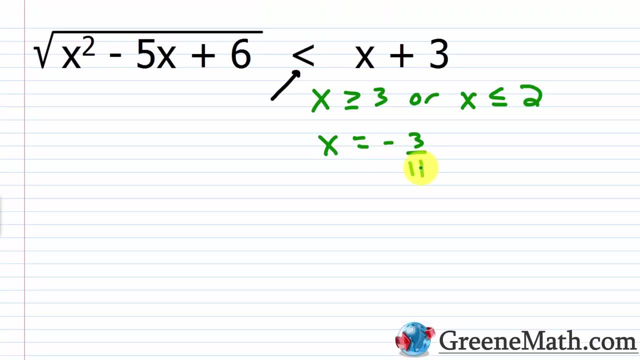 So I'm going to find that x is equal to negative 3 11ths. Okay, Negative 3 11ths. So let me erase everything, All right. So x is negative 3 11ths. That's our boundary. 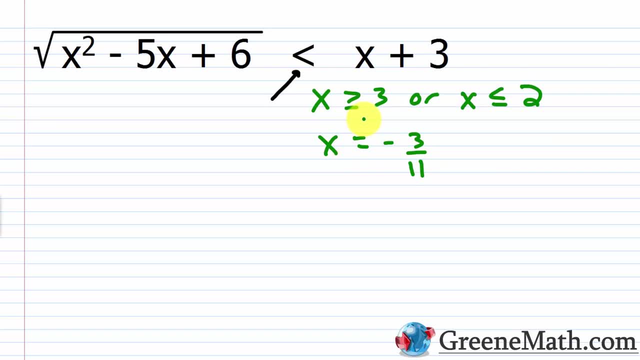 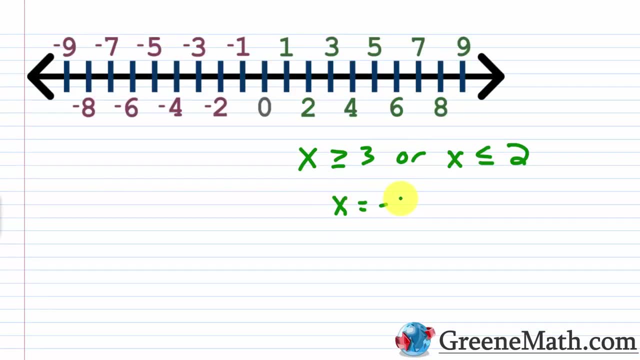 And again, the restrictions on the domain: x has to be greater than or equal to 3, or less than or equal to 2.. So let's go to the number line with this information. So again, we found that x was equal to negative 3 11ths. 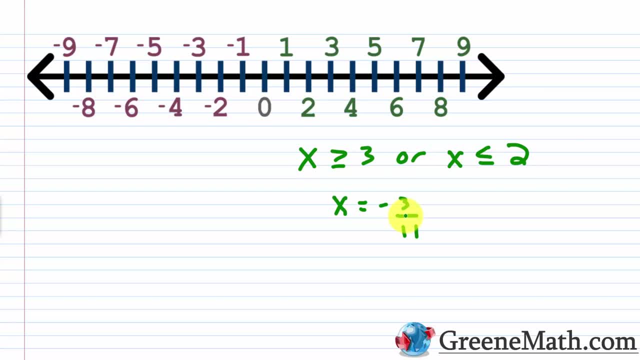 So that's our boundary. So negative 3 11ths As a decimal is a repeating decimal. It's negative 0.27, where that 2- 7 repeats forever. Okay, So if we wanted to put this on the number line, we could go about right here and just say that this represents negative 3 11ths. 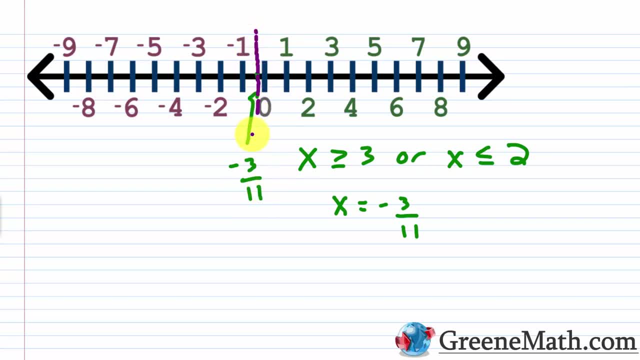 So I'm going to put a vertical line there, Okay. And then again, things need to be greater than or equal to 3. So I can put a vertical line here. and things need to be less than or equal to 2. So I can put a vertical line here. 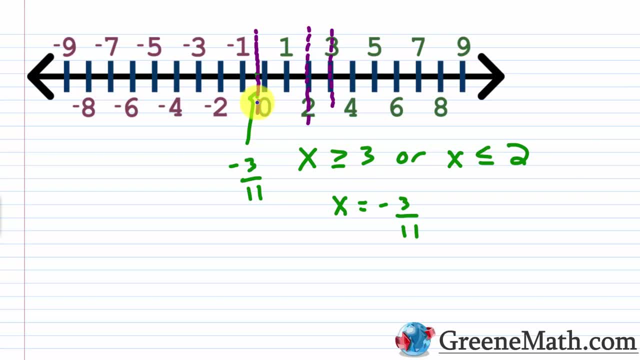 So if I call This to the left of negative 3 11ths, interval a, I could call between negative 3 11ths and 2 interval b, I could call between 2 and 3 interval c And I could call anything larger than 3 as interval d. 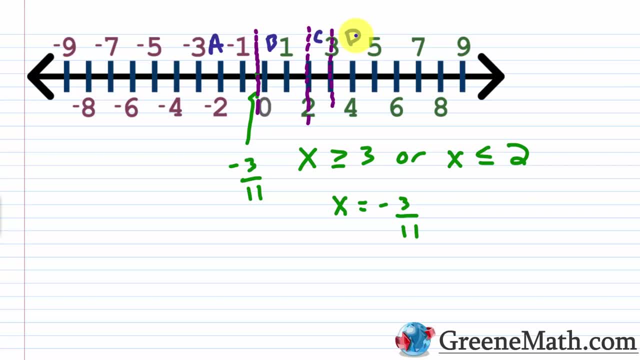 Now we know that things in interval c, okay between 2 and 3, don't work because they violate the domain. Okay, So I have a, b, c and d. Again, this is false. It doesn't work. 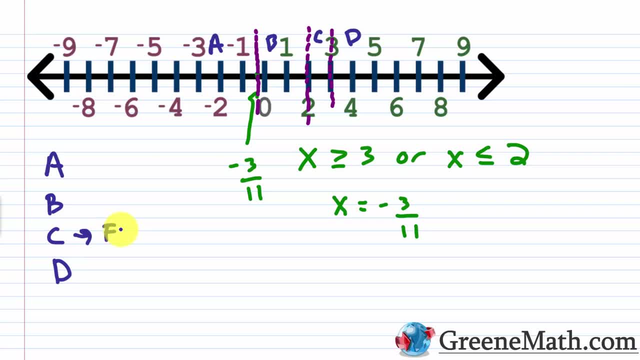 So let's choose a value in In interval a and see if that works. So again, our inequality was the square root of x squared minus 5x plus 6. Again, this had to be less than x plus 3.. So I'm going to pick a value of, let's say, negative 1.. 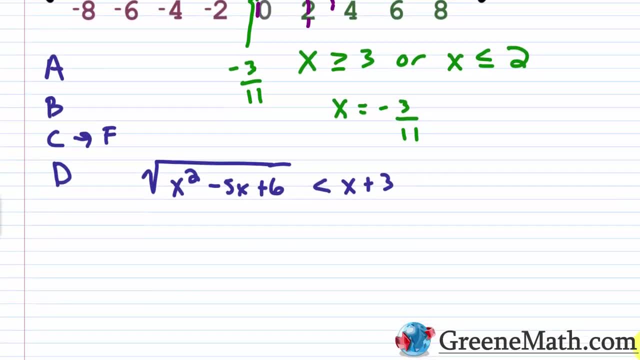 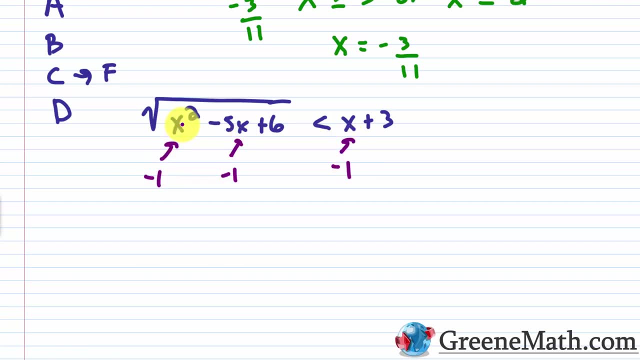 That's pretty easy to work with. So let me scroll down and get some room going. We'll come back up. So if I plugged in a negative 1 there and there and there, what would I get? Well, you'd have negative 1.. 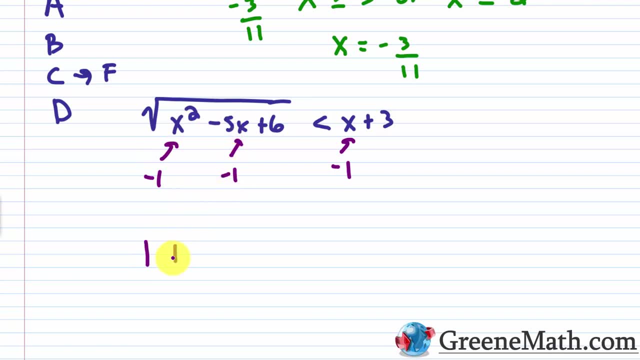 You'd have negative 1 squared, which is 1.. And then negative 5 times negative: 1 is plus 5.. And then you'd have plus 6.. So you'd have the square root of basically 12, right: 1 plus 5 is 6.. 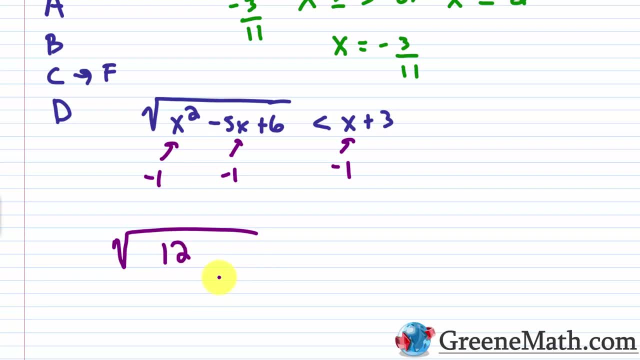 6 plus 6 is 12.. So the square root of 12 could be simplified as 2 times the square root of 3, right, Because 12 is 4 times 3.. 4 is a perfect square, So you could pull out the kind of 2 from that. 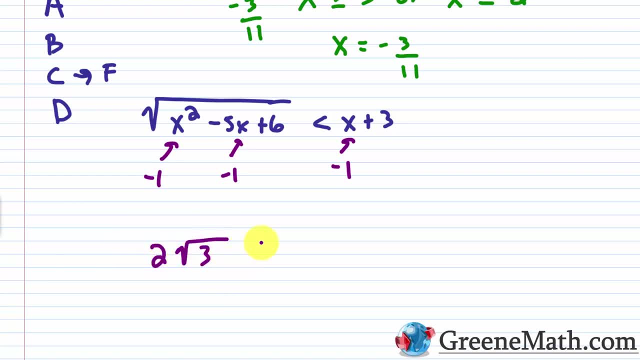 So you would have 2 times the square root of 3.. Okay, So this is less than negative. 1 plus 3 is 2.. Well, that's good. That's going to be false. If you do 2 times the square root of 3, you're going to get about 3.46.. 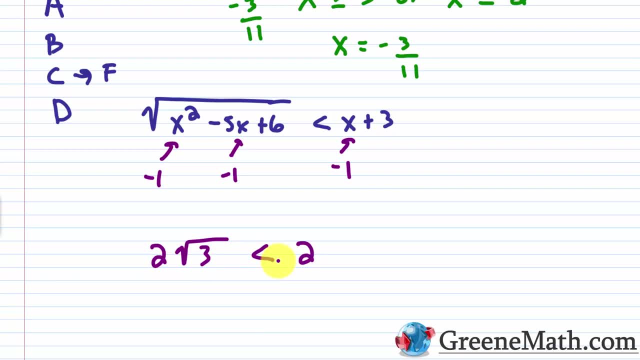 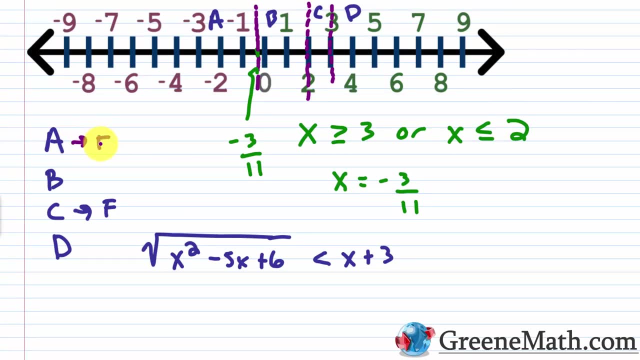 And that's clearly not less than 2.. So things in interval A don't work. Okay, Those are going to be false. So for interval A I'm going to put an F for false. Okay, What about things in interval B? 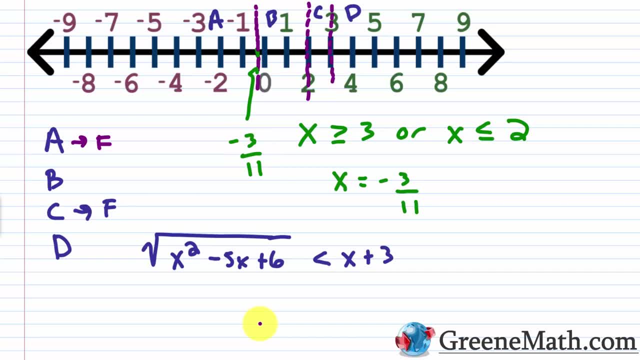 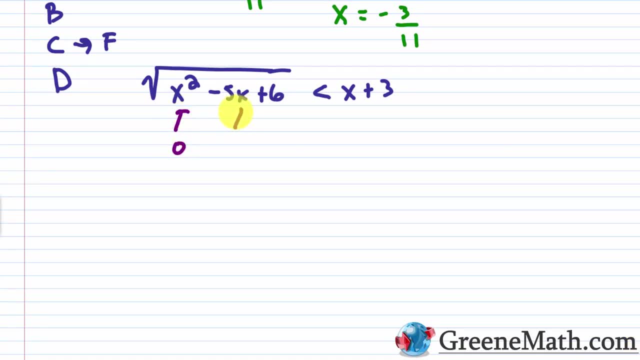 So this is between negative 3 11ths and again 2.. So let's think about the number 0.. That's easy to work with, So let's go ahead and plug that in for x. Okay, So 0 squared is 0.. 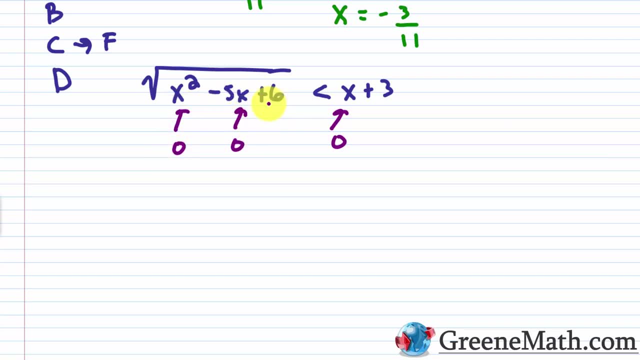 Then minus 5 times 0 is 0. So you basically just have your square root of 6 there, And that's less than If you have 0 plus 3, that's 3.. So the square root of 6 is again about 2.45,. you could say: 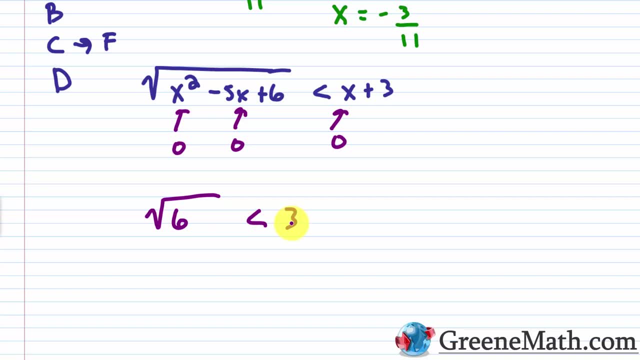 So that's going to be less than 3.. So values in interval B are going to work. So let's erase this. We'll come back up, So we'll put this one as true. Okay, So anything in interval B is going to work. 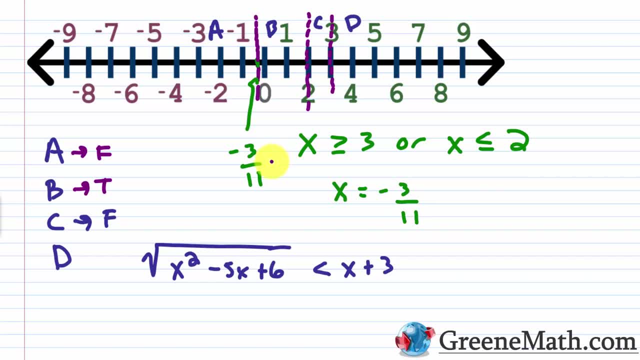 So anything in interval B is going to work. So anything larger than negative 3 11ths is going to work. Okay, Negative 3 11ths won't work. So that's going to include 2, because again 2 is in the domain. 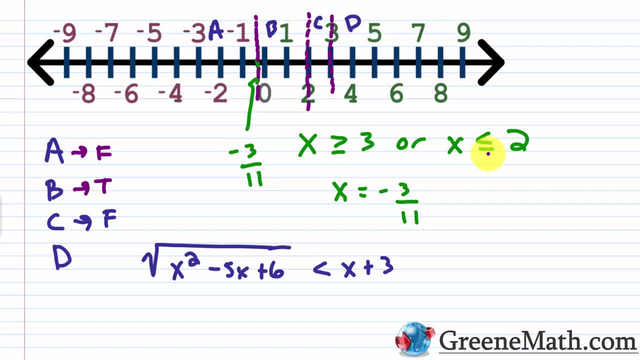 So we're good to go there. Now you can test something in interval D just to be safe, But essentially it's going to work Right, Because this is basically telling us that anything larger than negative 3 11ths is going to be a solution, with the exception of the numbers that violate the domain, which again, is anything between 2 and 3.. 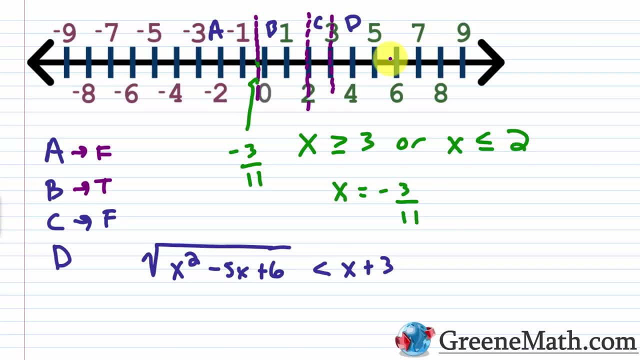 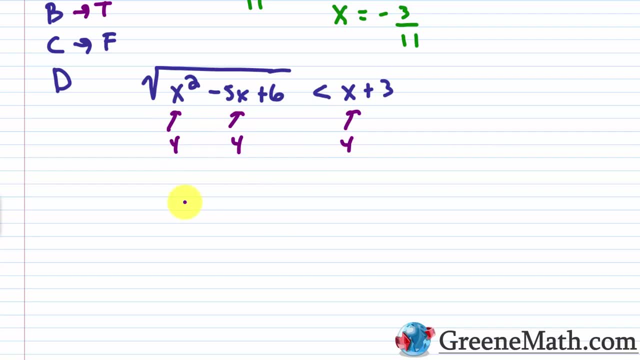 But let's take something from interval D. Let's just take 4 and see if that works, Just to be safe. So I plugged in a 4 there and there and there. What would I get? All right? So what I'd have here is the square root of 4. squared is 16.. 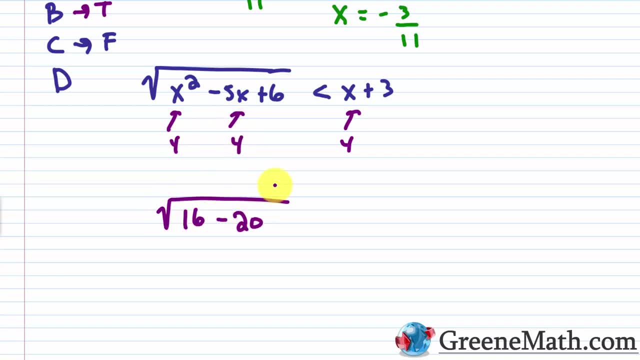 Then minus, you have 5 times 4,, which is 20.. Then plus 6. And this is less than 4 plus 3,, which is 7.. 16 minus 20 is negative, 4.. Negative: 4 plus 6 is 2.. 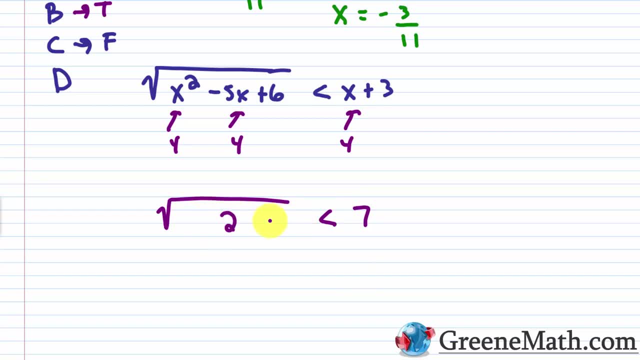 So you'd have: the square root of 2 is less than 7.. That's obviously true. So things in interval D will work. Okay. So let me erase all this. I'm ready to put our solution together, Okay. So, basically, anything to the left of negative 3 11ths doesn't work. 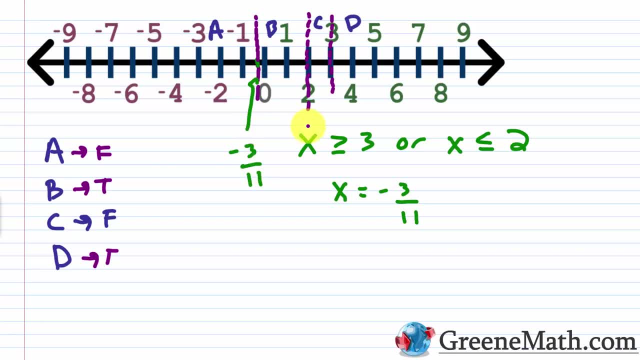 We know that Then anything greater than negative 3 11ths will work. But you have this restriction here, basically where between 2 and 3, it's not part of the domain, So you just have to exclude between 2 and 3..